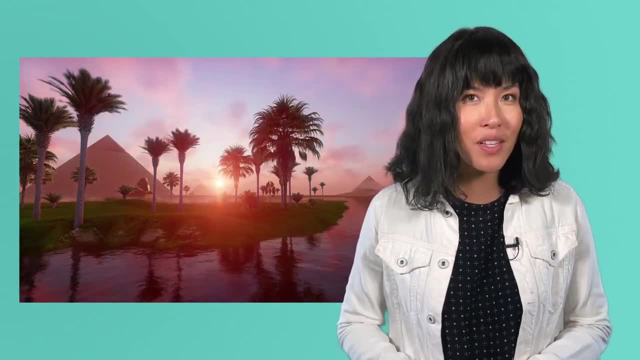 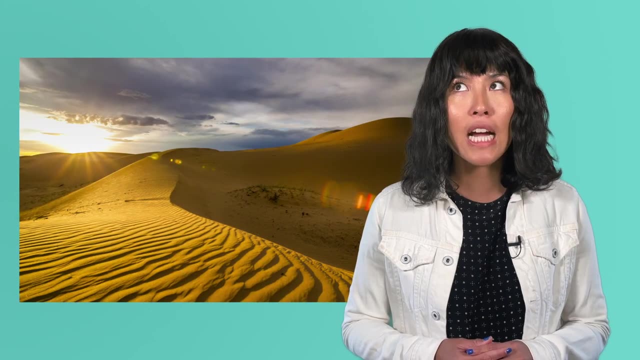 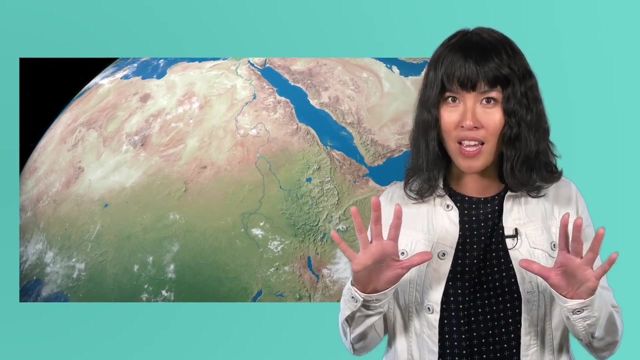 Ancient Egypt is one of the places where human civilization first really started to thrive, which might seem a little surprising considering that over 95% of the country is desert. But in between the expanses of the Sahara Desert is the Nile River. Now you might expect the banks. 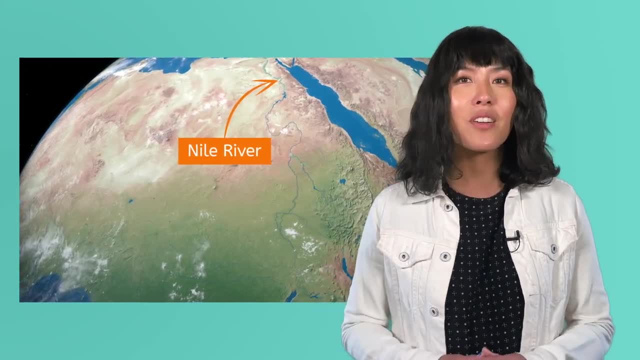 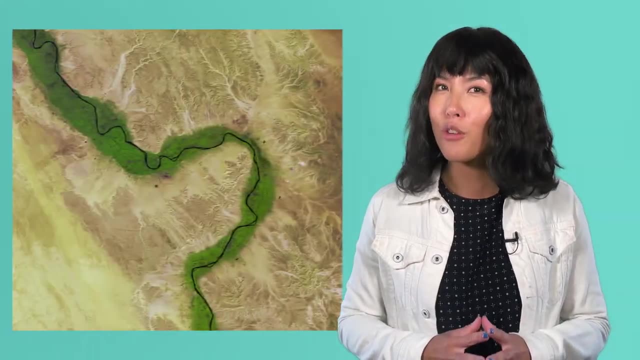 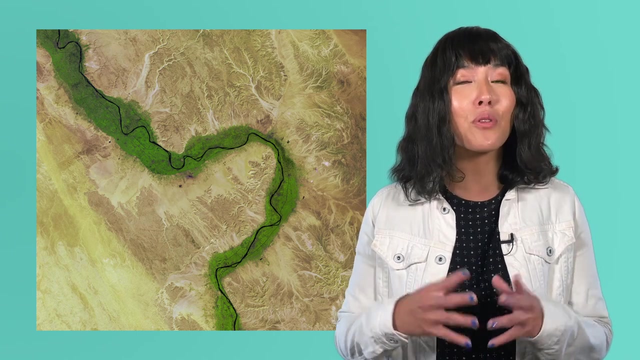 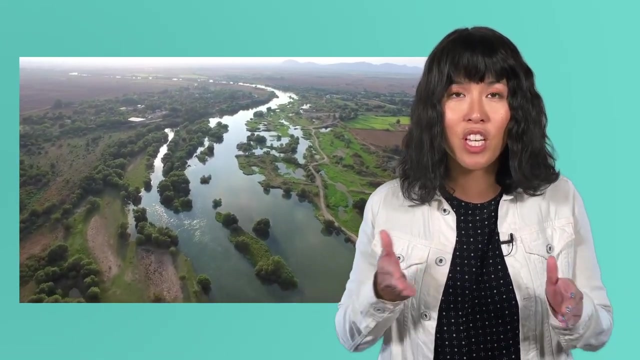 of this river to be more sandy desert, but it turns out. the Nile River is lined with miles of a lush green landscape. This fertile farmland is perfect for growing crops and is part of why the Ancient Egyptian civilization was able to thrive. So how did the area around this river become so different from the desert it runs through? 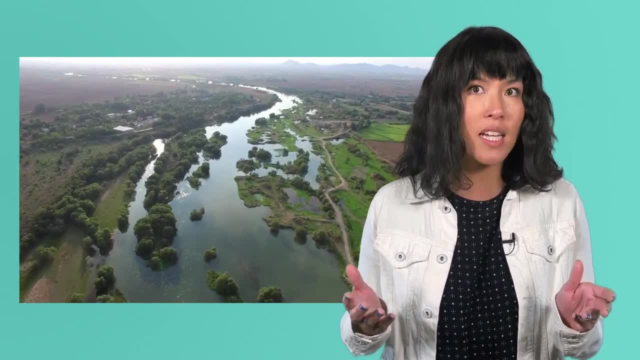 We know that soil is different from wet dirt or sand, so it's not like soil is different from sand. So how did the area around this river become so different from the desert it runs through? We know that soil is different from wet dirt or sand. 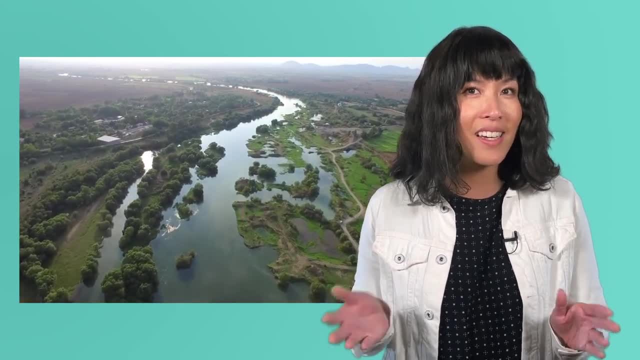 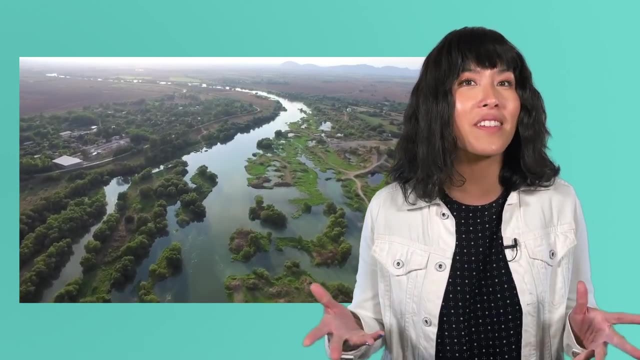 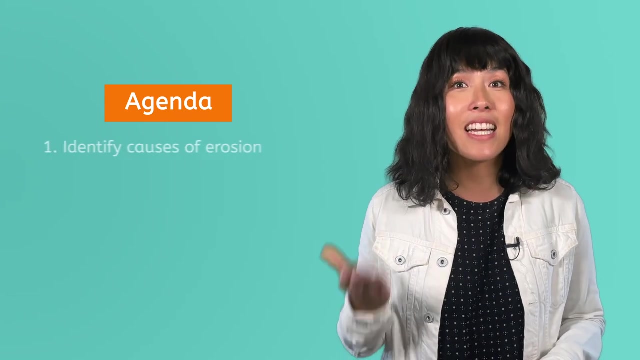 So it can't just be because of the river. right Today, we're going to explore the geological processes that made the Nile River Valley into flourishing farmland, even in the middle of the desert. By the end of this lesson, you should be able to identify causes of erosion, explain how. 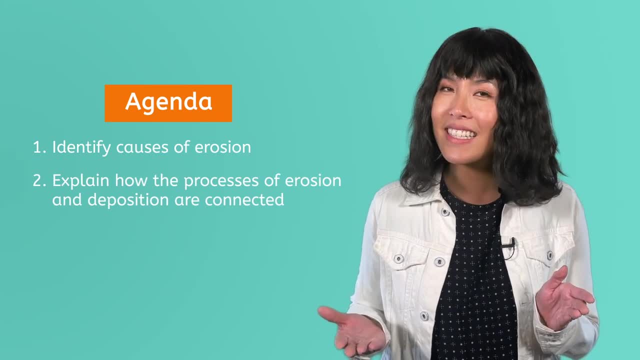 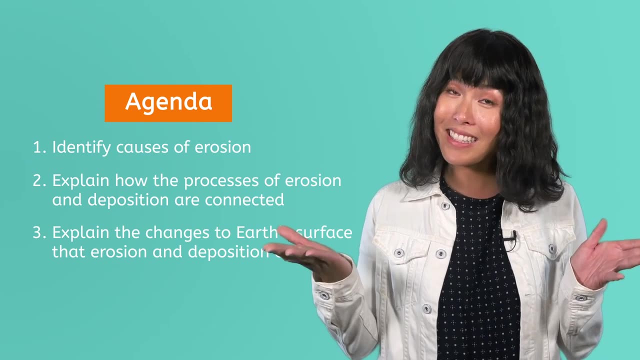 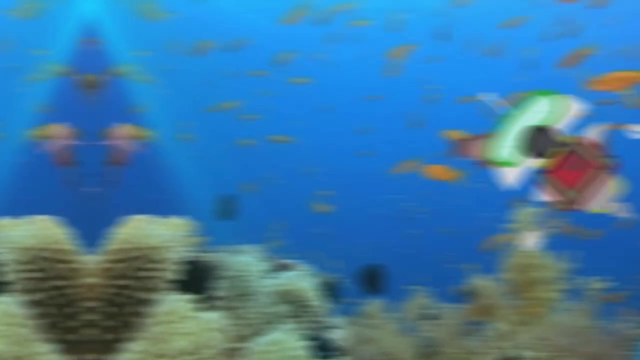 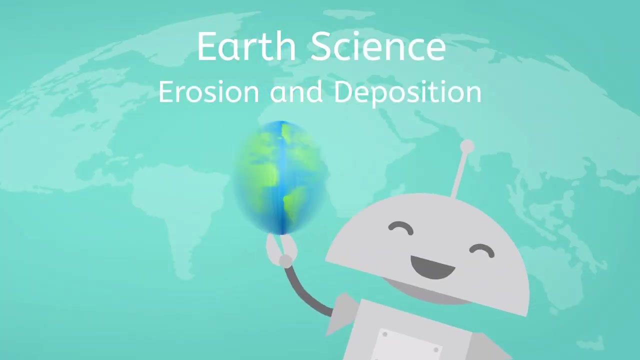 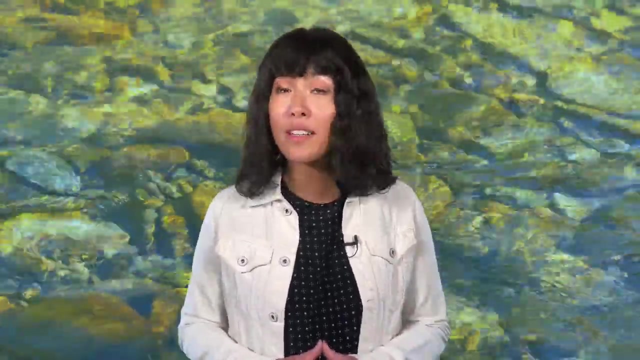 the processes of erosion and deposition are connected and explain the changes to Earth's surface that erosion and deposition cause. Let's get started. In our last lesson we learned about the processes of weathering and erosion. Weathering is when natural forces break rocks down. 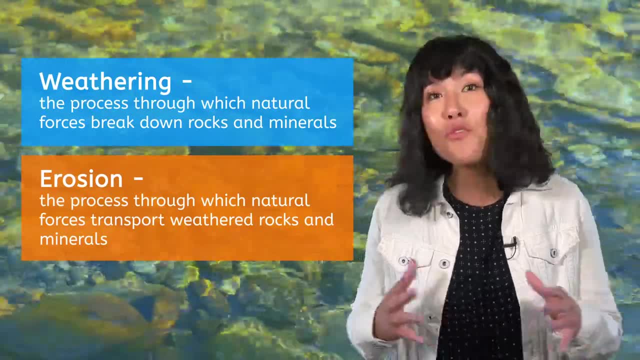 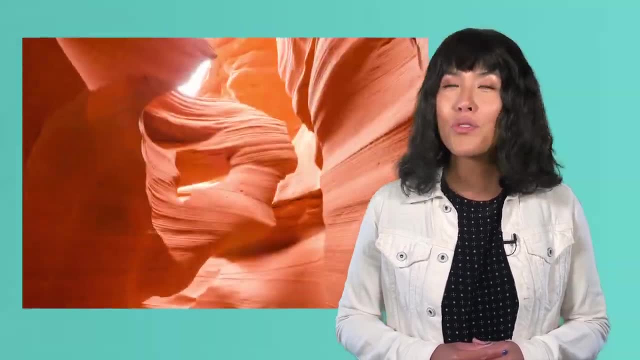 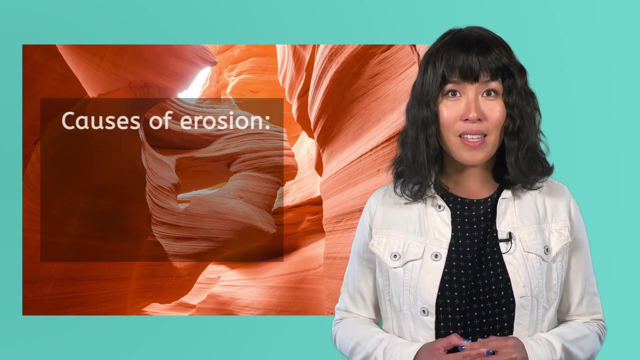 And erosion is when these forces move them across the Earth's surface. For now, we're going to mostly focus on erosion. Erosion is a natural process that is part of the rock cycle and there are a few different ways it can happen. 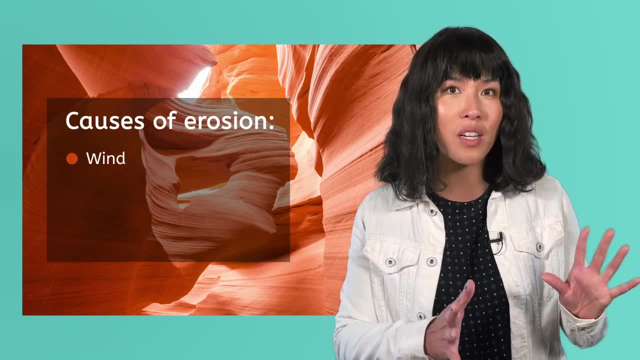 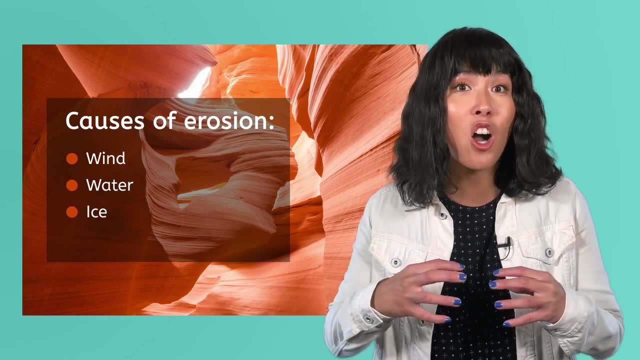 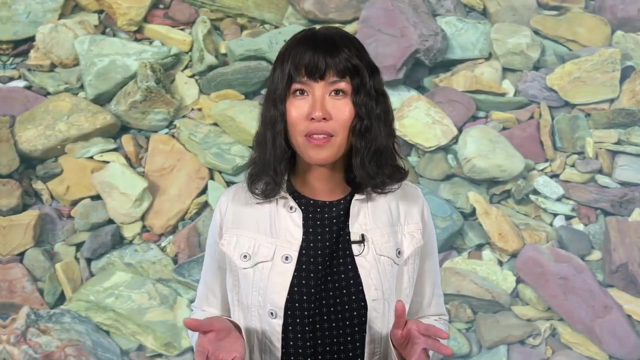 The main causes are: when wind blows rocks around, when moving water from rainfall or streams carries rocks away, when ice carries rocks along with a glacier, or when grass falls, Gravity simply makes rocks fall to somewhere else. Now you might be thinking: okay, so a couple of pebbles move around, what's the big deal? 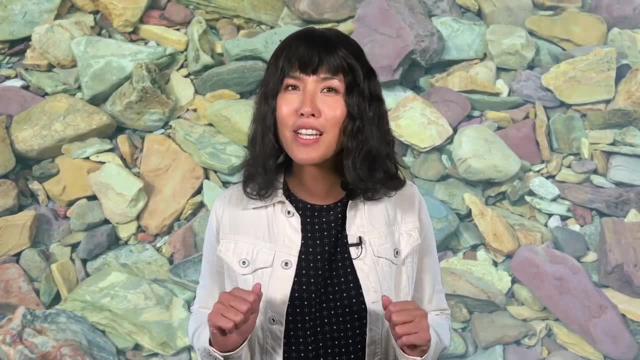 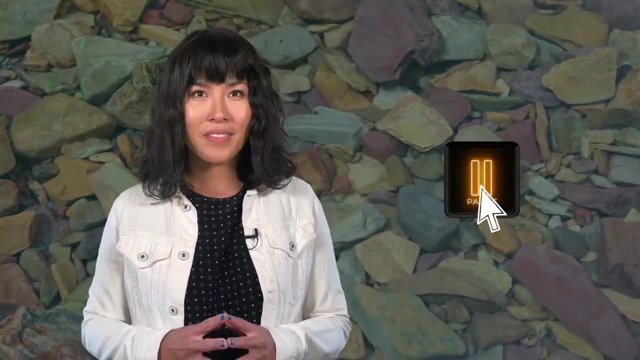 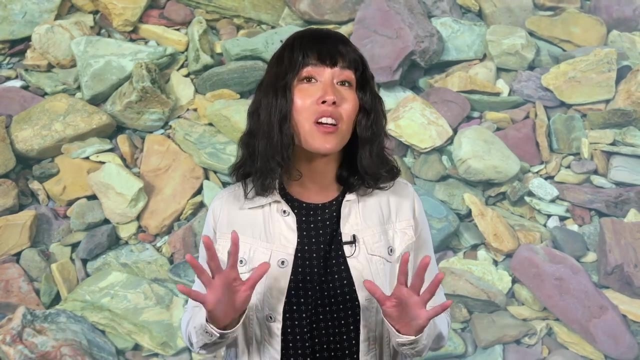 about erosion. Pause the video here and write down why you think erosion might be an important geological process in your guided notes. Remember, when we describe geological processes, we're talking about things that are slow but constant. Let's say, erosion results in a storm. 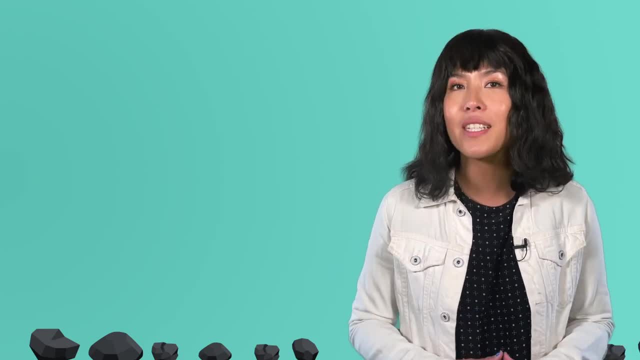 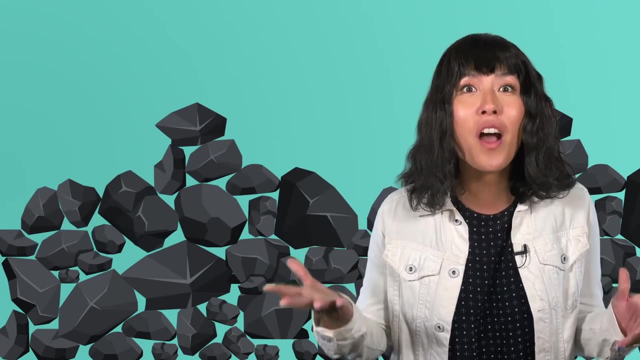 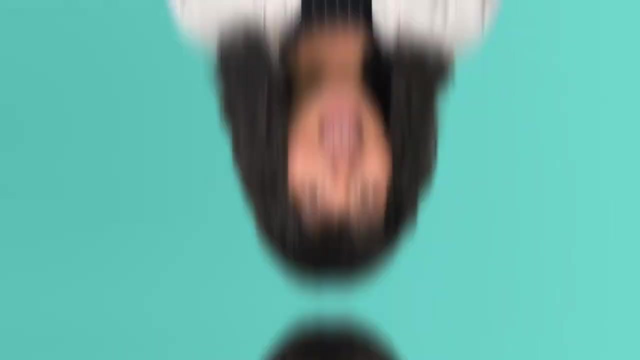 Erosion results in only five or six rocks moving off a mountain every day. At the end of a year that's about 2,000 rocks. After 100 years it's 200,000 rocks. After a long enough time it can literally move mountains. 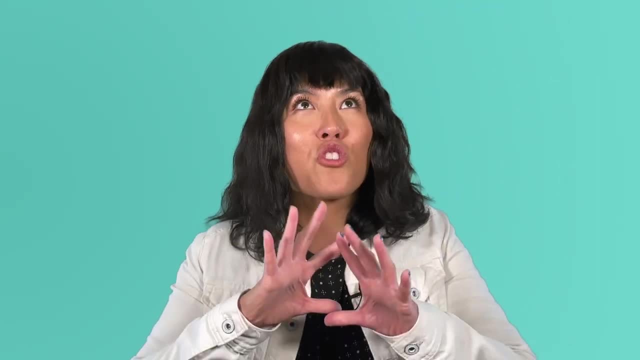 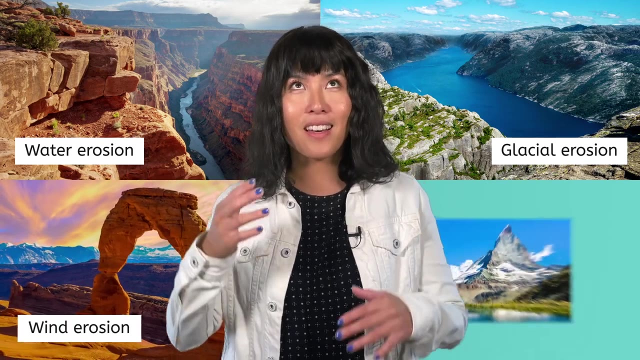 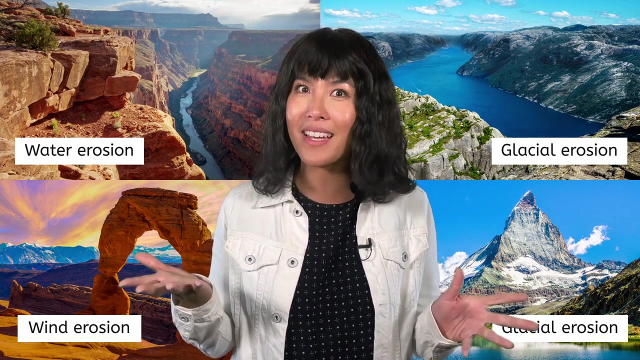 Different kinds of erosion have played a part in shaping some of Earth's most unique land forms, like the Grand Canyon, the Norwegian Fjords Arches National Park and the Matterhorn. So we've seen what happens when erosion removes rocks and sculpts landforms like these. 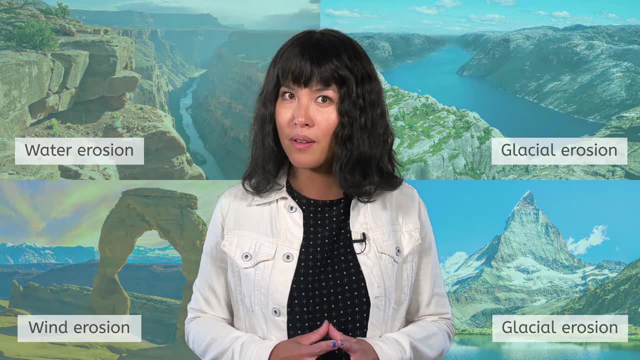 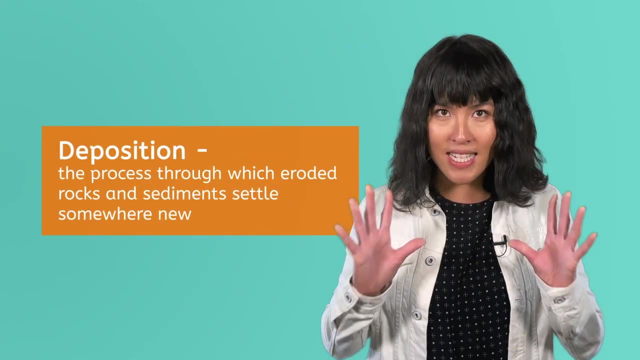 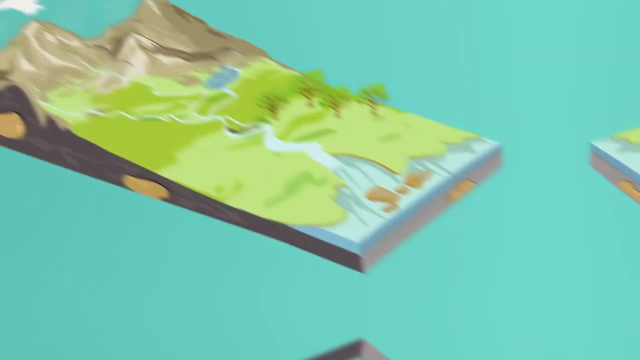 But the question is: where do they end up? That's where our next process comes in. Erosion is followed by another process called deposition, which is when eroded rocks and sediments are deposited and settle somewhere new. So, while erosion shapes the Earth's surface, by carving away the earth's surface, erosion 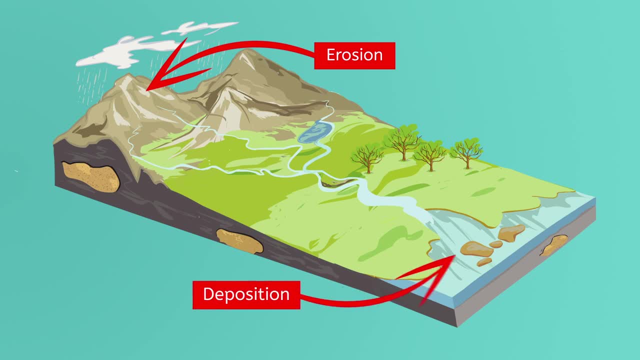 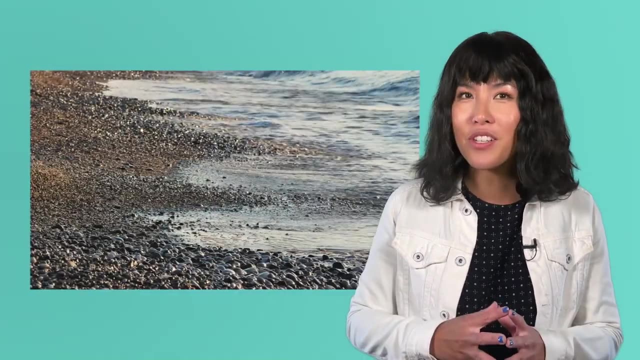 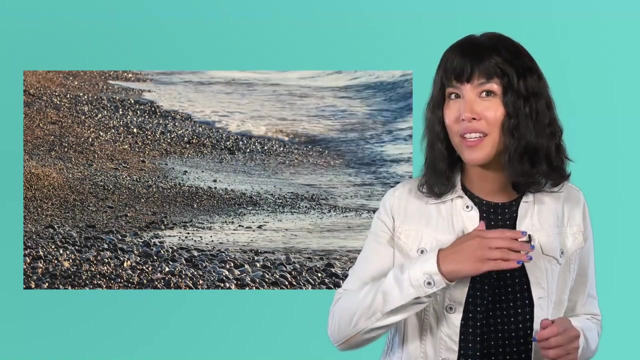 is also a process of deposition When erosion shapes the earth's surface. erosion shapes the earth's surface by carving away pieces of the land. Deposition shapes it by dropping off rocks that create new landforms. Beaches are created by the deposition of sand, rocks and shells that were eroded by the ocean. 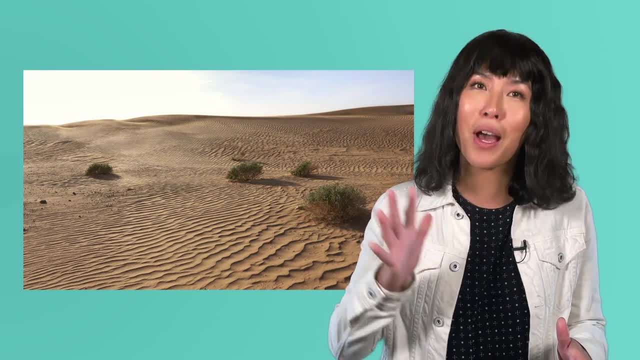 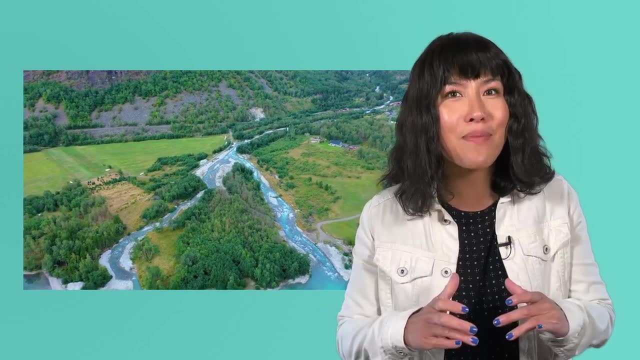 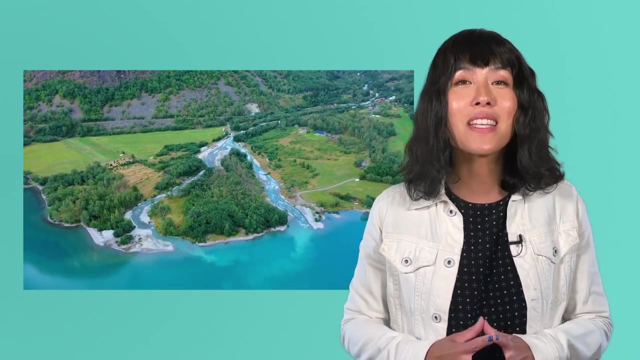 Sand dunes are rolling hills of sand deposited by wind, And river deltas are triangular landforms made when a river deposits the sediment it has eroded before it has been eroded. So in this case, we're talking about sand deposits emptying into another body of water, which, it turns out, is what makes the Nile River Delta. 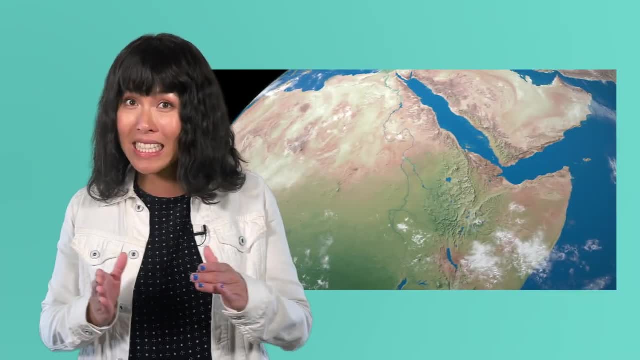 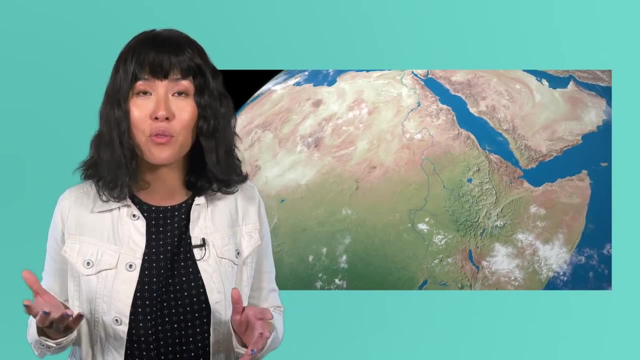 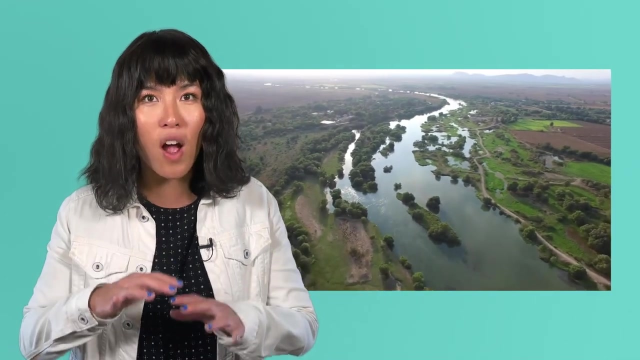 so perfect for growing crops. After winding its way through Africa for over 4,000 miles, the Nile River erodes tons of rocks and minerals At the end of its journey. when the Nile is emptying into the Mediterranean Sea, it deposits these rocks and minerals along the River Delta.